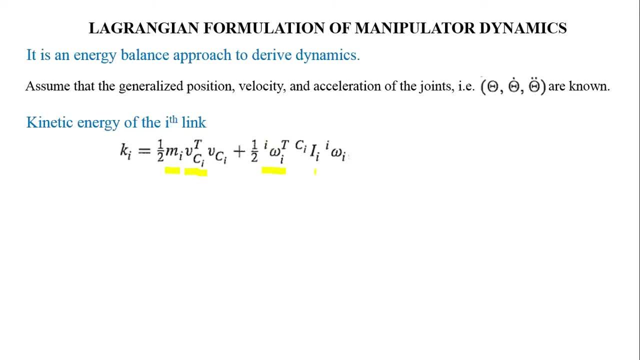 on the same link. i is denoted by i, omega i. this c, i, i i denotes the inertia tensor of the ith link with respect to the ith i plane, which has the origin at the center of mass of the ith link. now, potential energy of the ith link has been denoted by the term ui and it is equal to minus. 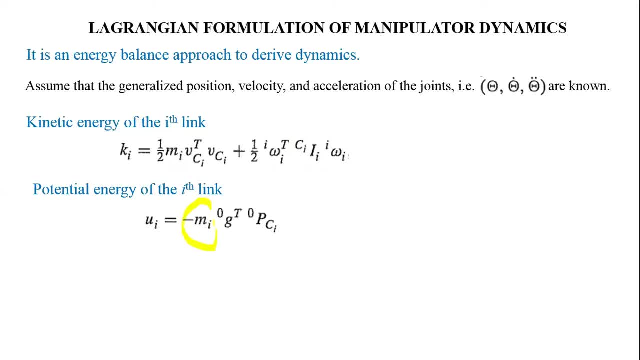 m, g, s, where m is denoted mass of the ith link, denoted by the mi, and the gravitational vector is noted by g 0, which is gravitational vector with respect to base reference frame, and 0 pci denotes the position of the, the position of the center of mass of the ith link with respect to zero reference frame or base. 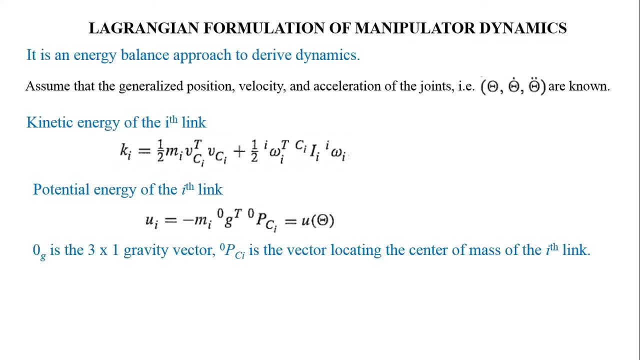 reference frame. the potential energy is a function of position, so ui can be written as u, theta, and the kinetic energy is a function of theta and theta dot, so it can written as k theta, theta dot. next, the lagrangian variable is defined, and the lagrangian variable is denoted by this term. 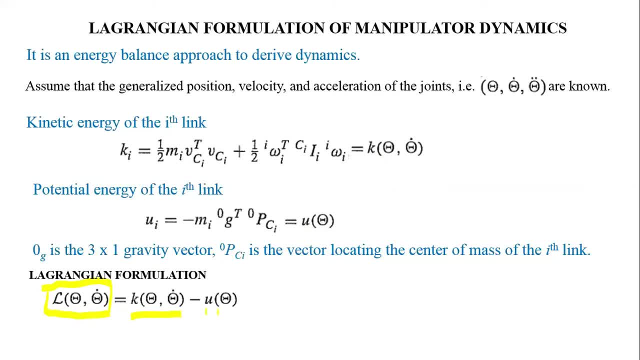 and this lagrangian variable is equal to kinetic energy minus potential energy. if we make a differential equation in this form, by taking partial derivative of the lagrangian variable with respect to below theta, dot and theta, then we can find out the torque variable after substituting the expression of lagrangian. 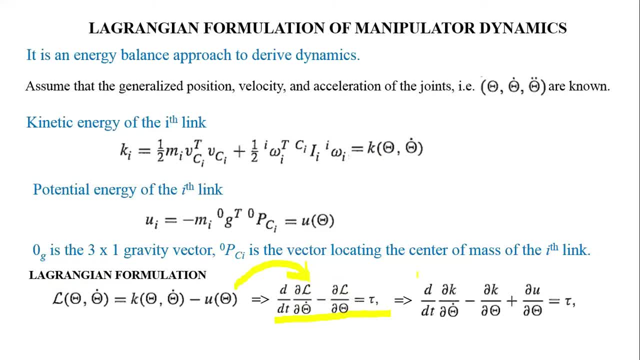 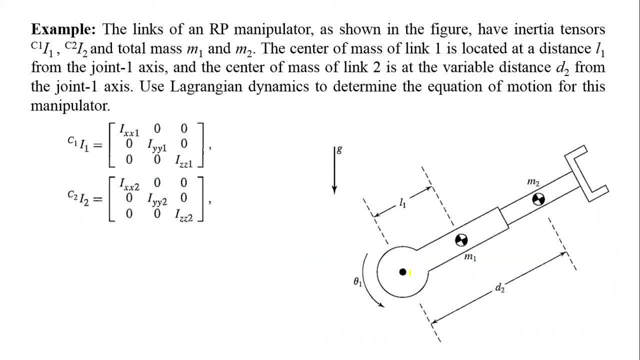 variable. we can find out this expression, this differential equation. let's derive the dynamics of this manipulator shown in the figure. it is a rp manipulator and it has inertia tensors. this and this. the matrices are shown over here. total mass of the link one and link two are m1 and m2. 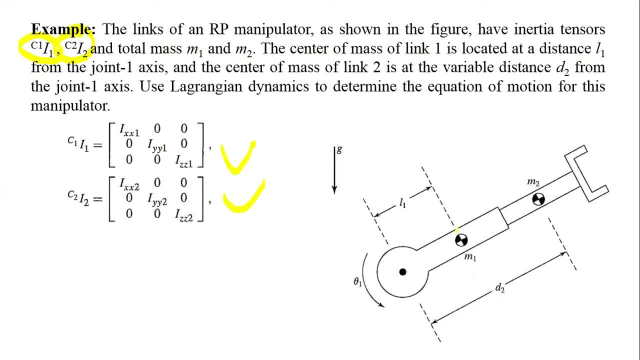 the center of mass of link one is located at a distance l1, so this is the center of mass of the first link and the joint to one x is. and the center of mass of link two is the variable between d2 from the joint one x, so this is the location of second centre of mass of the ring. 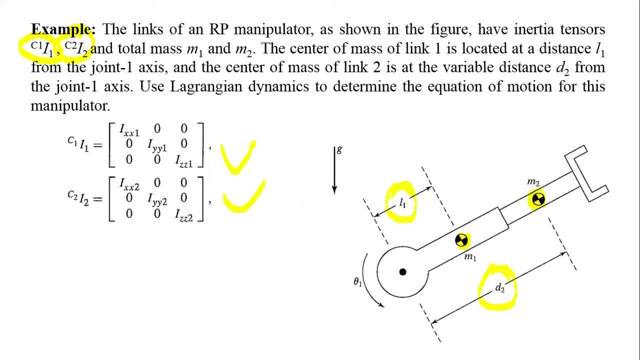 and this length is variable, but this length is sometimes. now we need to use lagrangian dynamics to determine the equation of motion for this manipulator. the total kinetic energy of this manipulator produced by the first link will be equal to half mass of first link m1 into v square. v square means v is equal to. 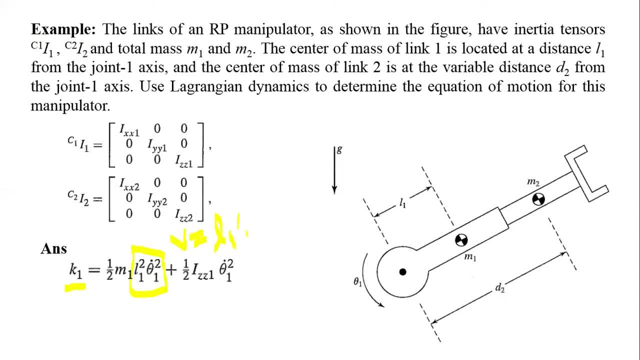 l1 theta 1 dot. so if we take the square, then v square will be equal to l1 theta 1 dot square. so we will get half mv square plus half i omega square. omega is omega is theta 1 dot. similarly, the kinetic energy produced by the second link can be: 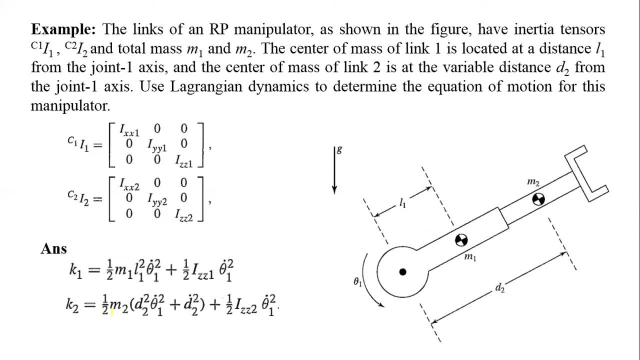 expressed in this form, and here the half mass of the second link into velocity of center of mass that is equal to d2 theta 1 dot, d2 theta 1 dot. that means this velocity- d2 theta 1 dot- plus kinetic energy produced by this velocity, that is 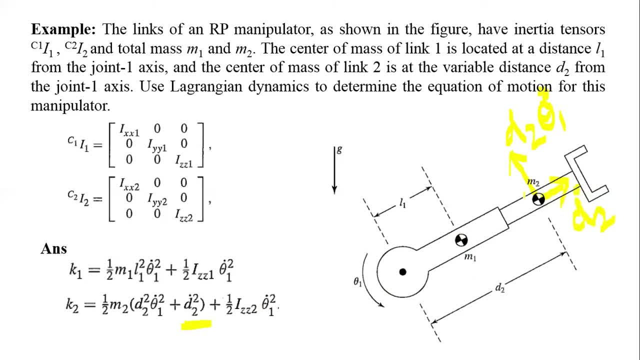 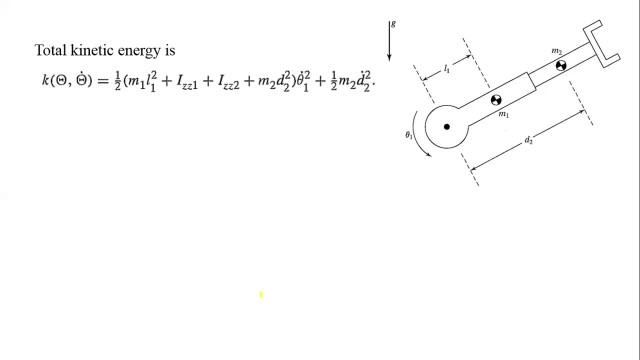 delta, d2, dot, plus kinetic energy produced by the angular rotation of this link, that is, r to i, omega square, total kinetic energy of this manipulator will be equal to k1 plus k2 and the expression will be like this: now, potential energy. potential energy produced by the first link will be: 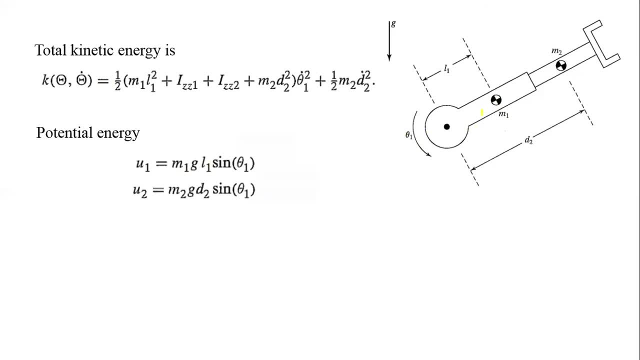 m1 g, m1 g vertically downward plus i, that will be l1 times theta 1. due to m2 v weight into d2 sine theta 1, total potential energy will be equal to u1 plus u2 and we'll get this expression now. if we take partial derivative of kinetic energy with respect to theta dot, then we'll: 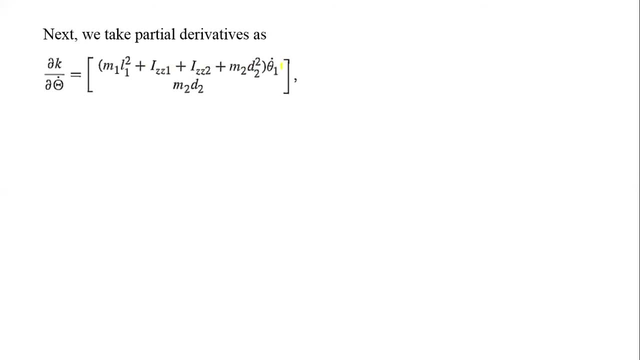 get this matrix. so this matrix is a two by one matrix. so these two elements are obtained by this differentiation. so the first element of this matrix has been obtained by taking partial derivatives of total kinetic energy with respect to eta 1 dot, and the second element has been obtained by taking the 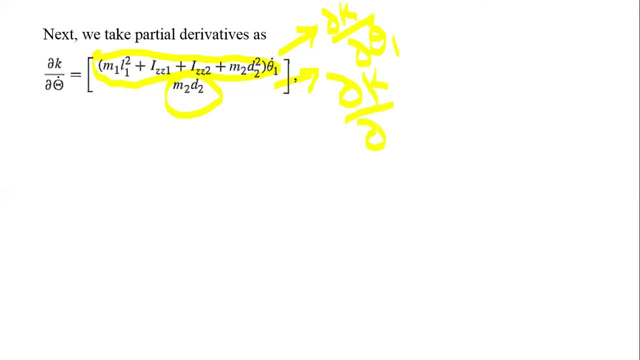 partial derivative of total kinetic energy with respect to d2 dot. similarly, if we take partial derivative of kinetic energy with respect to theta, we will get this matrix. and if we take partial derivative of total potential energy with respect to theta, we will get this matrix. now, if we substitute these partial 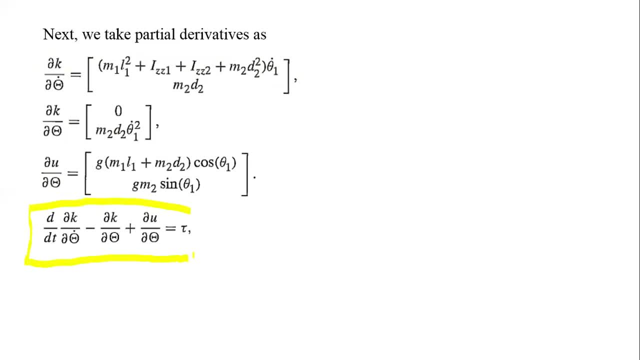 derivatives into the expression of lagrangian formulation. then we can find out the expression of torque acting on the first link and torque acting on the second link, and the expressions will be like this: tau 1 and tau 2. so this tau 1 will be obtained by using this energy. 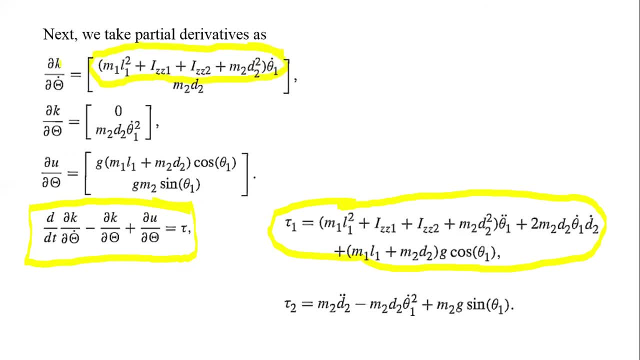 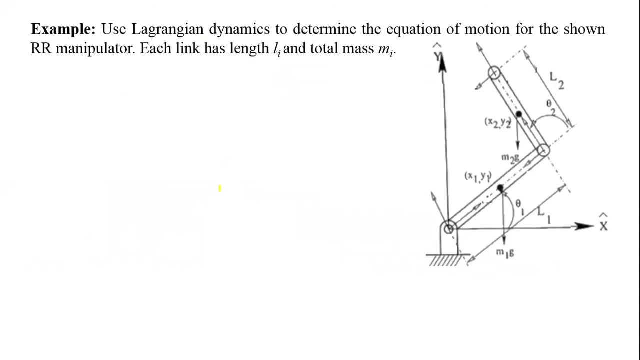 element of the equation del k by delta dot, and this equation and this expression and this tau 2 will be obtained by using the second element of the matrices. let's understand the lagrangian formulation with help of another example, and this is example of rr manipulator, where each link has 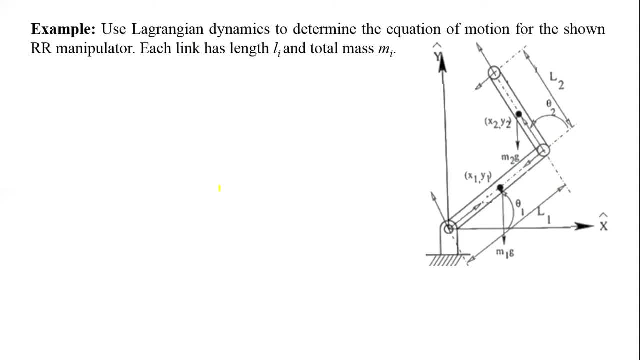 each link has length length l i. that means the length of the link is l1 and the length of the link is l2. total mass of first link is m1 and the second link is m2. here the length should be capital l5. that means the length of first link is capital l1 length length of second link is capital l2. now 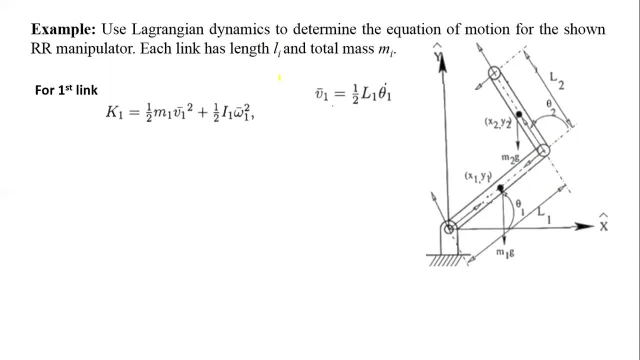 the first link, the expression of kinetic energy will be like this: where v1 is half l1, theta 1 dot and omega 1 is equal to theta 1 dot. inertia tensor can be calculated with the help of this expression that we have derived in our previous lecture. so this is the inertia tensor for a cylindrical link with respect to: 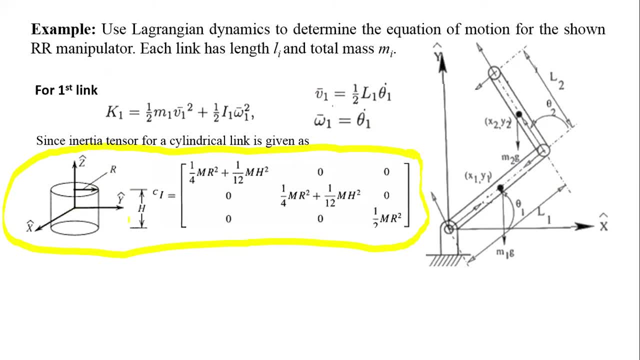 the frame located at the center of mass of the link, so ci, that means inertia. tensor with respect to this c reference frame will be equal to this matrix and the moment of inertia of the first link about its, about its center of mass, will be equal to. i1 is equal to 1 by 12 m1 l1 square plus 1 by 4. 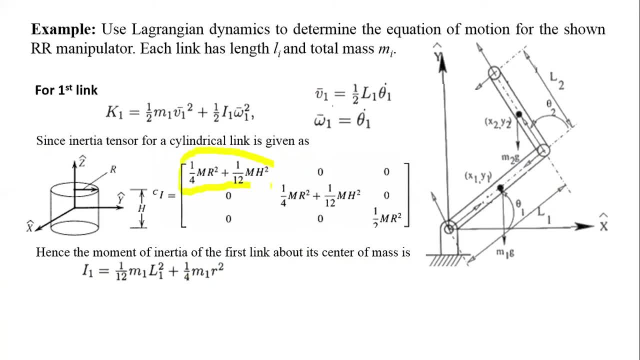 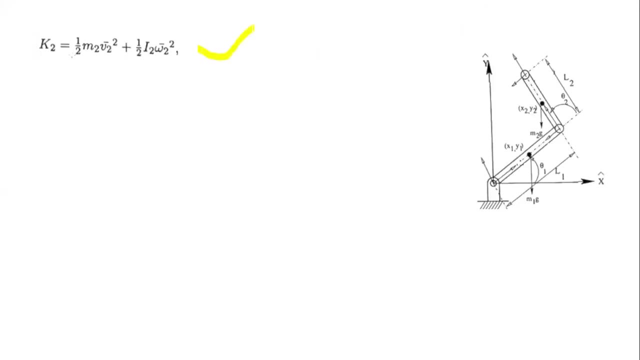 m1 r square. that means we are taking this type of expression after substituting this inertia expression in the kinetic energy expression we get: k1 is equal to this equation and k2 is equal to this equation. where v2 will be equal to x2 dot square plus y2 dot square, omega 2 will be equal. 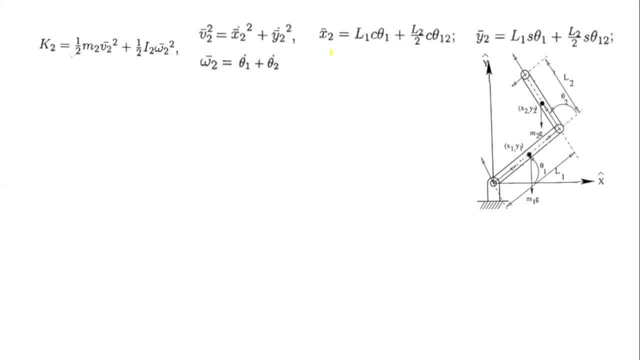 to theta 1 dot plus theta 2 dot. x2 can be derived using this expression and y2 will be equal to theta 1 dot plus theta 2 dot expression and y2 will be obtained from this expression. and these expressions are just denoting the geometry of the robot manipulator. Similarly, we can find out the inertia expression. 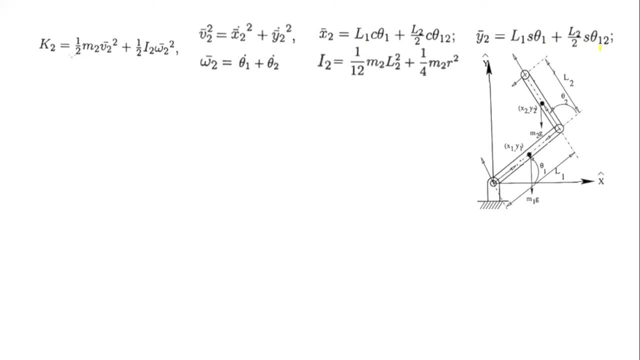 for the link 2, and this will be equal to. I2 is equal to 1 by 12 m2 L2 square plus 1 by 4 m2 R square. After substituting the expression of x2- y2 in this equation, we get the expression: 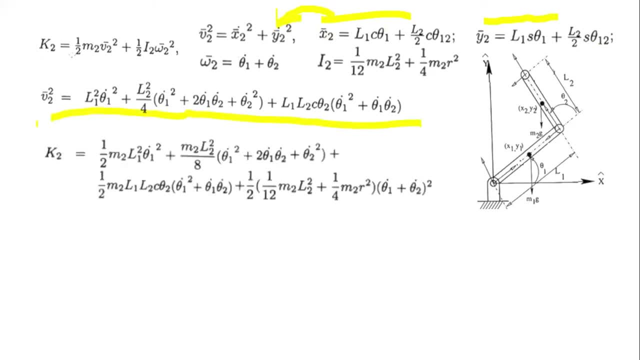 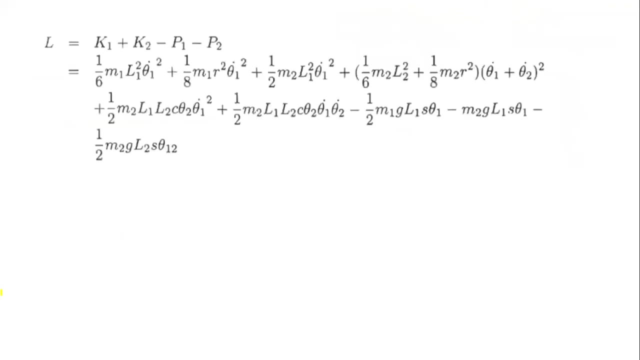 of velocity like this, and once we substitute this velocity equation in k2, we get this expression of k2.. Now the potential energy of the first link will be equal to half m1, g, L1, sine theta, 1 and p2 will be equal to this expression. The Lagrangian variable will: 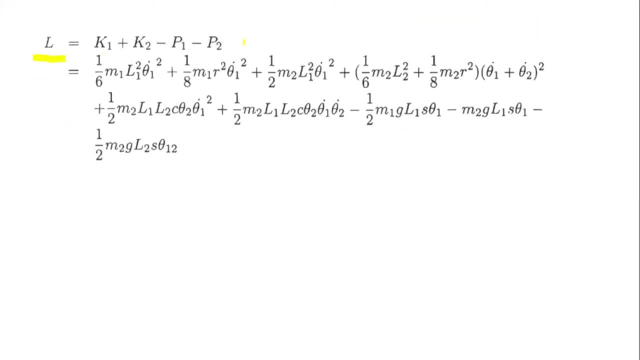 be L equal to k1 plus k2 minus k1 plus p2.. Just substitute the expressions of k1, k2, p1, p2 and take the derivative of Lagrangian variable with respect to theta 1 dot and again its derivative with respect to theta 2.. 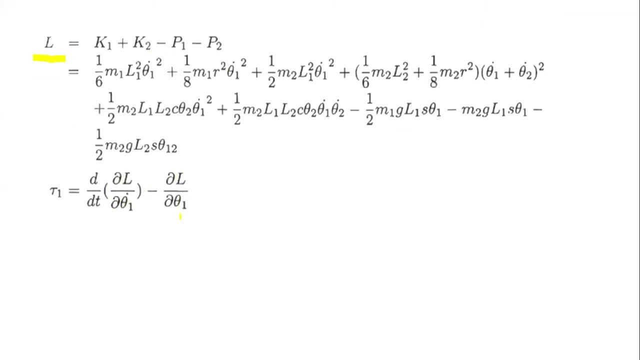 Then subtract this del L by del theta 1.. That means partial derivative of Lagrangian variable with respect to theta 1, and finally we will get the expression of tor acting on first link and second link. So here you can see the partial derivative of Lagrangian variable. 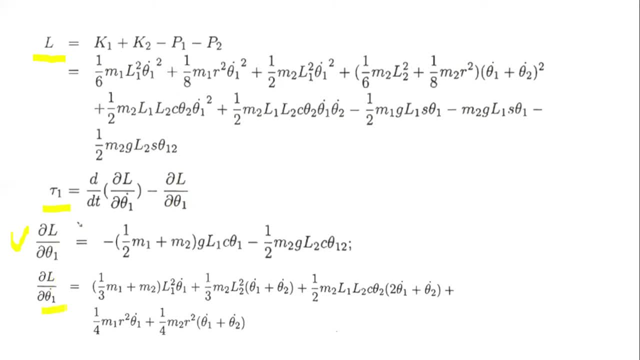 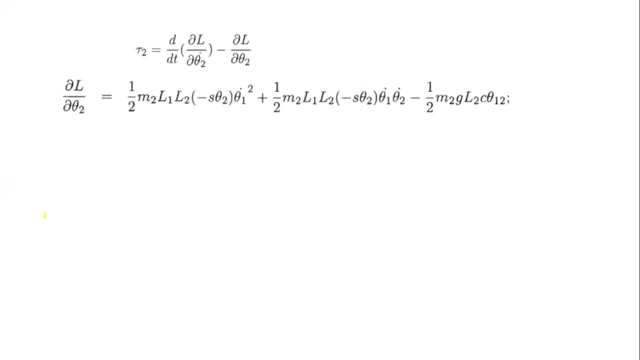 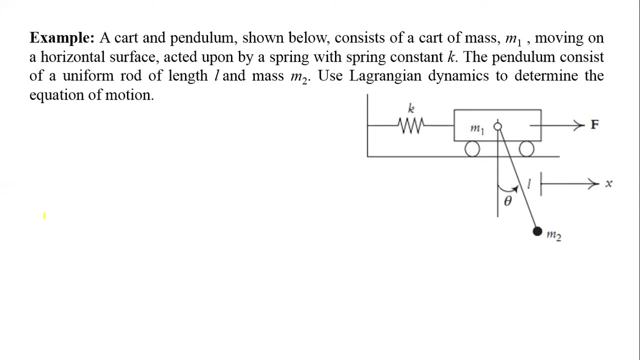 with respect to theta 1 and partial derivative of Lagrangian variable with respect to theta 1, dot and this derivative, and after substituting we got the expression of tau 1 and tau 2.. Another example: It is a cart and pendulum shown in this figure. It consists of a cart. 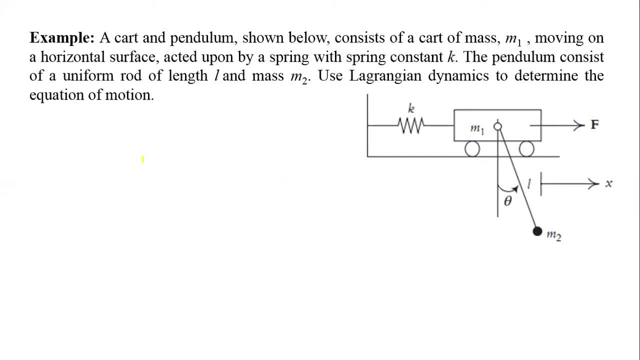 of mass m1, moving on a horizontal surface acted upon by a spring, with the spring constant k. The pendulum consists of a uniform rod, So this is a uniform rod, and the length of this rod is L and mass is m2.. So the mass of the pendulum rod is m2.. We have to use 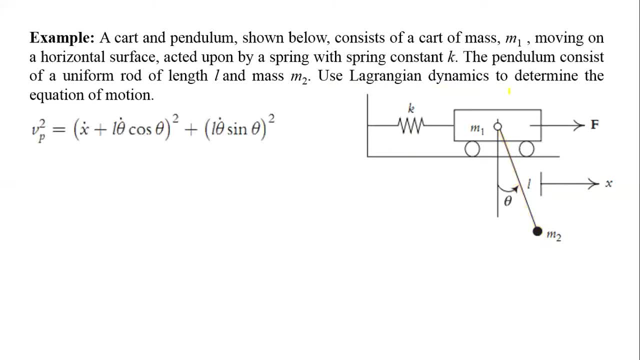 Lagrangian dynamics to determine the equation of motor. So the velocity of pendulum can be derived using this expression and the kinetic energy of cart will be equal to half m1 x dot square. Kinetic energy produced by pendulum will be equal to half m2 into Vp square. So this is Vp square. Next, kinetic energy will be: 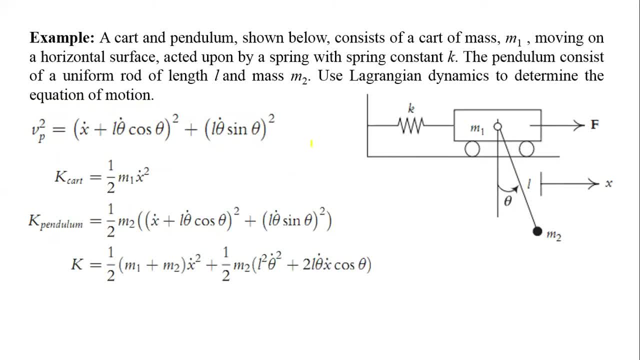 equal to k cart plus k pendulum. So the value of k cart is equal to half k cart plus k pendulum And the expression will be like this: Potential energy will be equal to half k- x square. the potential energy produced by the. 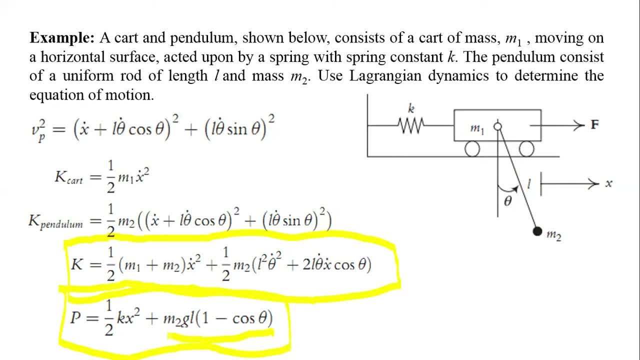 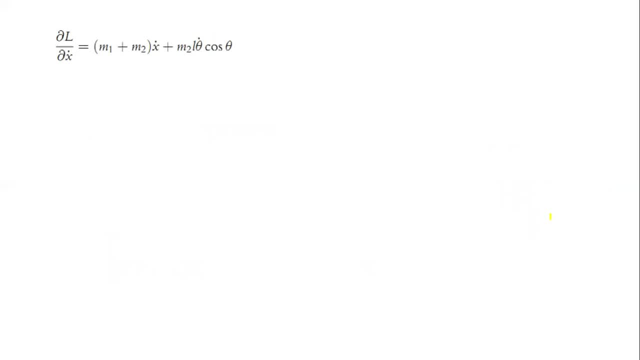 spring plus m2, g l 1, minus cos, theta, that is potential energy of this pendulum. Take partial derivative of Lagrangian variable with respect to x dot and using these partial derivatives- partial derivatives- we can find out the force acting on the cart and the torque acting on. 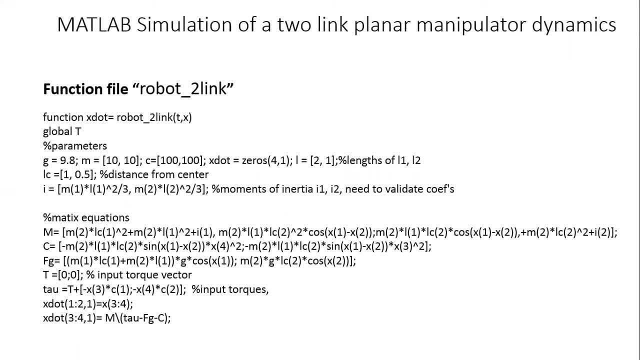 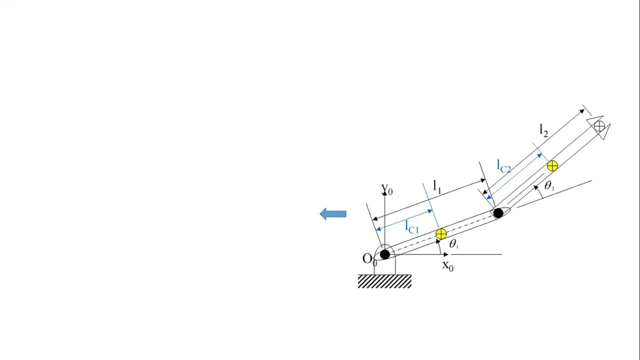 the pendulum. The code for simulating two-link planar maneuverability dynamics is written here. You can use it directly and simulate the responses in the MATLAB framework. The forward dynamics has been simulated for the initial condition of all the positions, like theta1 and theta2 are kept zero initially and the torque is zero-zero. 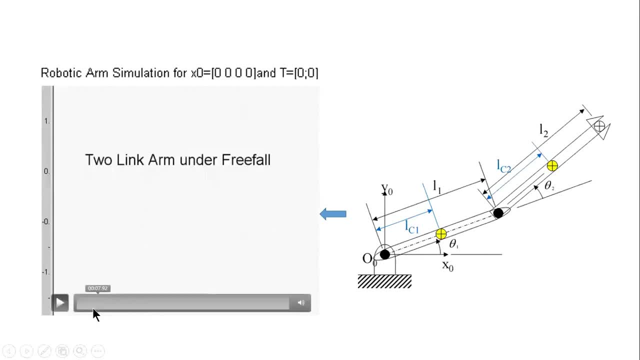 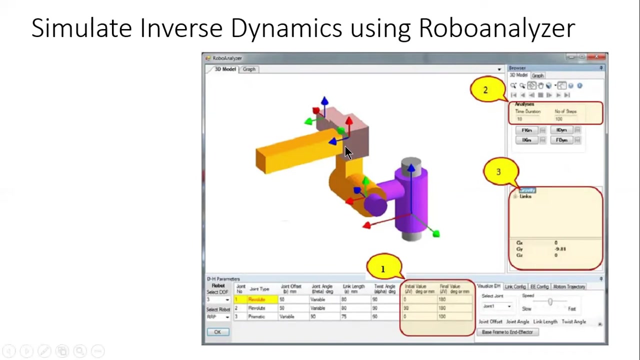 That means the simulation will be done for three fall conditions. The simulation response looks like this: Another very popular product for analyzing robot behavior is RoboAnalyzer. So you can simulate the robot behavior using this RoboAnalyzer and for simulating inverse dynamics or any of the equations we use for simulating inverse dynamics, we use following: 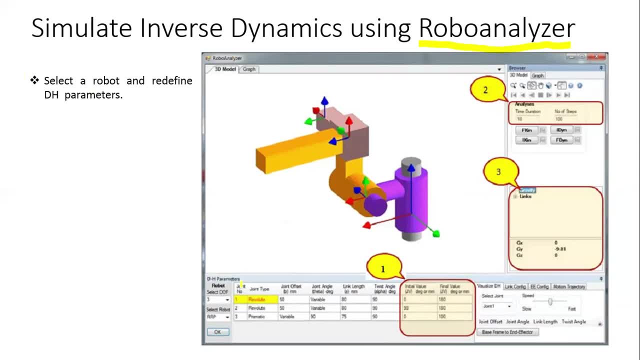 steps. First of all, we select the robot and redefine the pH parameters. the pH parameters are entered in this, And then we follow the following steps. The first step: we set the initial and final values of joint variables in this place. Then we set time, duration and number of steps for the simulation. 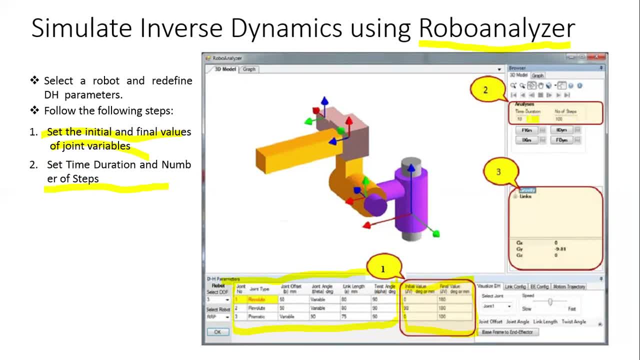 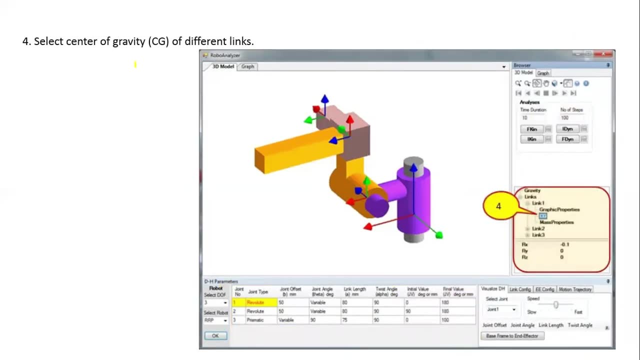 And the time duration of simulation is 10, and this 10 seconds will be simulated in 100 number of steps. Then we set gravity in SI units or, entering the gravity values, select this option of gravity. Then we select center of gravity. We select center of gravity of different links by clicking on this option, CD and enter. 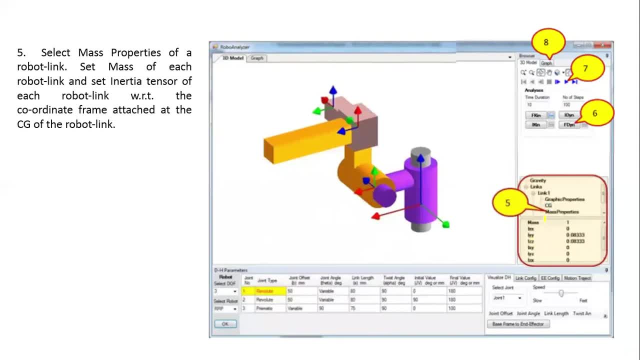 the values RX, RY and RJ, Then select the mass properties of each link, and the mass properties of each link means the masses of links and inertia tension for each link with respect to coordinate frame at the center of gravity of the robot link. Then click on F dynamics. 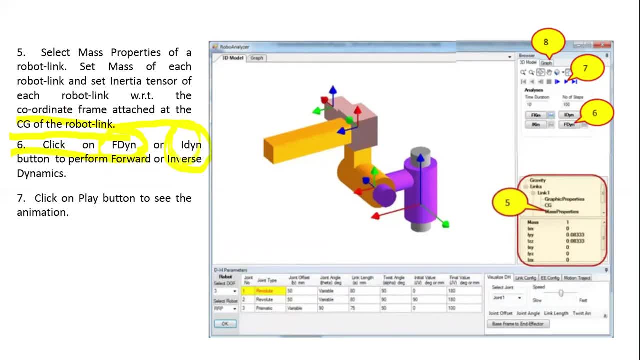 If you want to calculate forward dynamics or click invert, I will show you how to do it. I will select IDYN. you want to calculate the inverse dynamics, where it will find the options IDYN and FDYN? Here is the option. 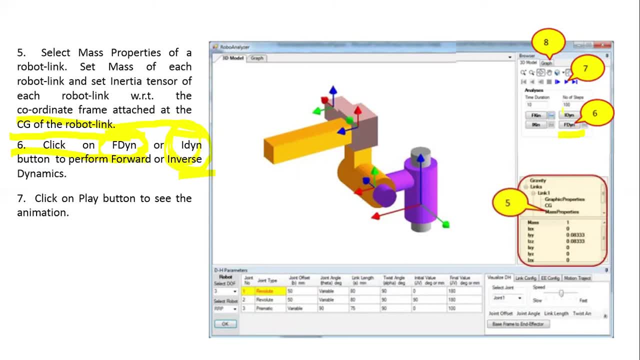 So if you correct this FDYN, you will get the forward dynamics. If you click on IDYN, then you will get the inverse dynamics behavior of this robot. Then next step is click on play button. So click on the play button and this robot behavior will be animated in this space and 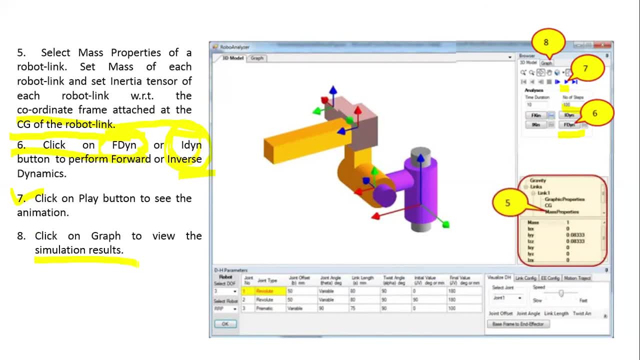 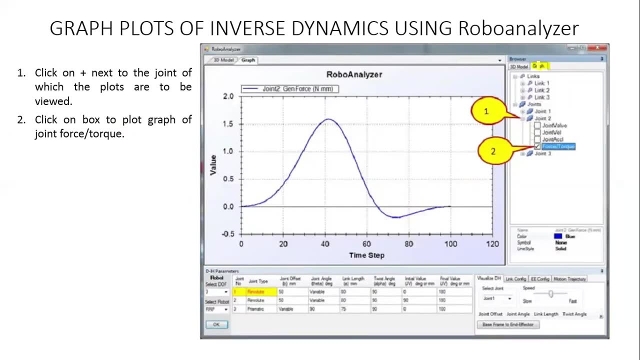 if you want to activate this, to see the graph, then go to this tab: graph. so once you click this graph tab, you will find this type of window and then this option, the plus next to the joints. so here, in this case, the robot is consisting of three joints: 21, 22, 23- so you can get the simulation results for each joint. so till now, 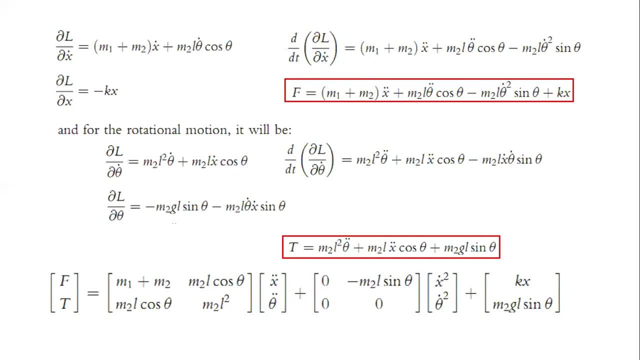 the application of lagrangian mechanics on a manipulator having maximum two degree of freedom has been demonstrated, but what will be the procedure of applying lagrangian mechanics on any kind of manipulator having degree of freedom one, two, three, four or any number? so in